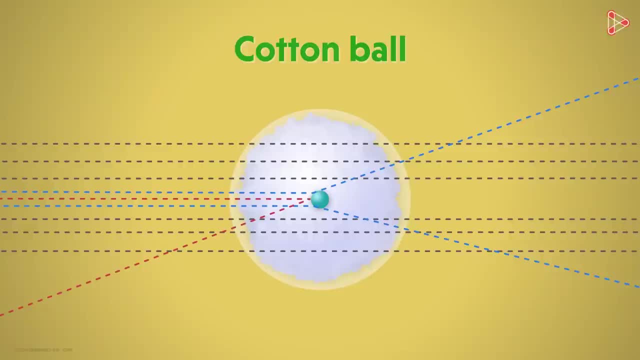 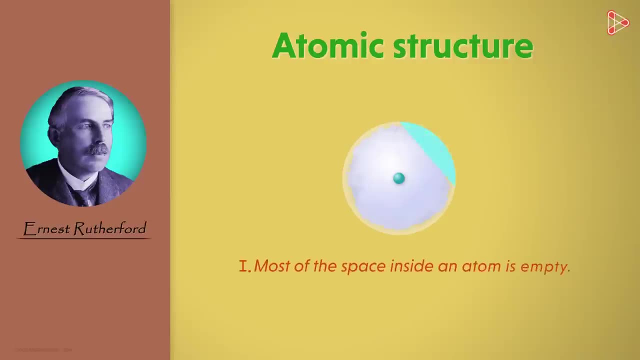 So very few bullets will bounce back. This is analogous to what Rutherford had inferred about the atomic structure. His first conclusion was that most of the space inside an atom is empty. This is because most of the alpha particles go hope. so particles could easily pass through the atoms and hit the detector straight. 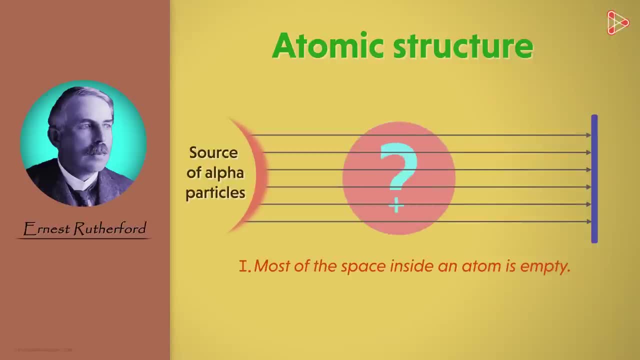 Now, if most of the space is empty inside an atom, then where is the positive charge located? Well, that's the second conclusion. The positive charge is compactly packed in a tiny entity. This occupies an extremely small space inside the atom. Now, why did he think so? 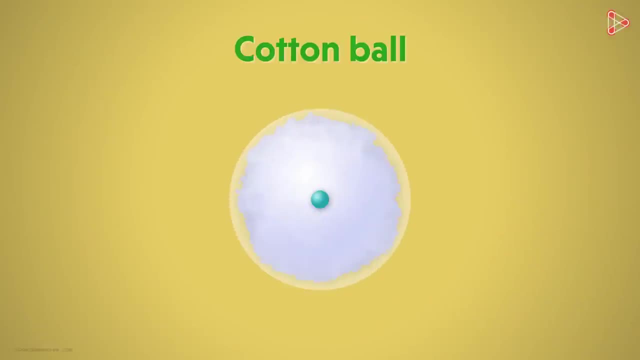 Let's go back to our cotton ball and bullet example. Can you recall the second and the third case? Yes, the bullets get deviated on hitting the tiny sphere of the edge and they will rebound when they hit the centre. Same explanation holds true for this. 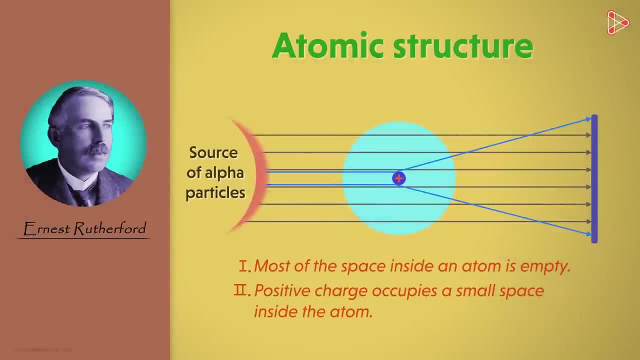 A few alpha particles get deviated. That means there is a possibility that these hit the edge of the positive centre. Yes, and one more possibility is that they get deviated because the positive centre repels the alpha particles as they are also positively charged. 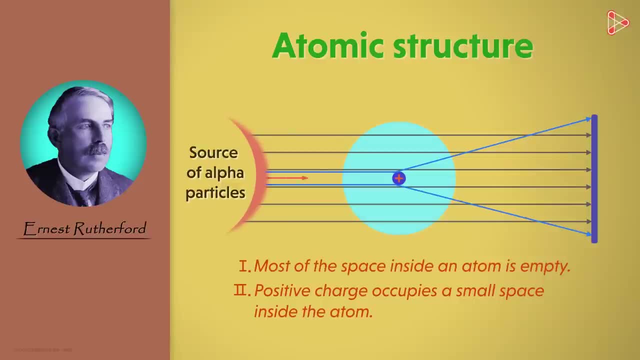 Also a very small number of alpha particles rebounded. That means there is a possibility that these alpha particles had directly hit the positive centre. But since the number of these rebounding particles is too small, it explains that the volume occupied by the positive centre is also very small. 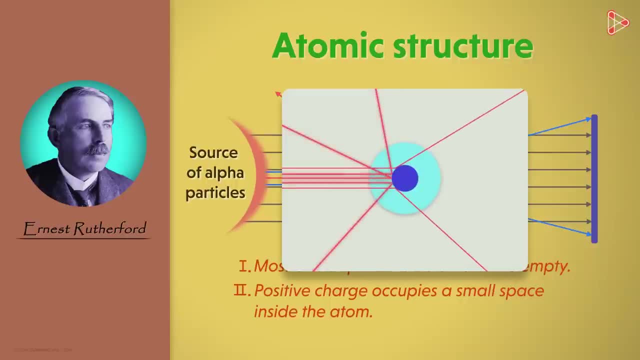 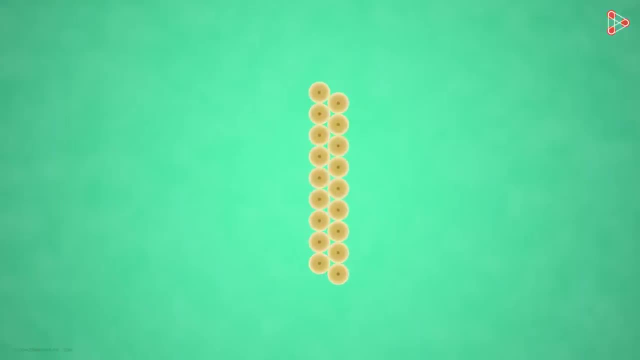 If the space occupied would have been big enough, then the number of alpha particles bouncing back would also be greater. So let's say there are gold particles. So let's say there are gold particles in the foil. He found that most of the rays pass straight through the atoms. 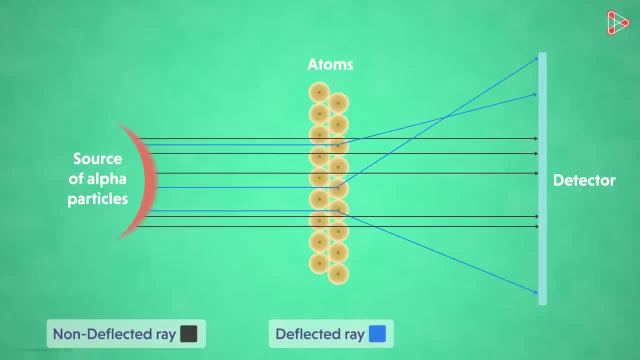 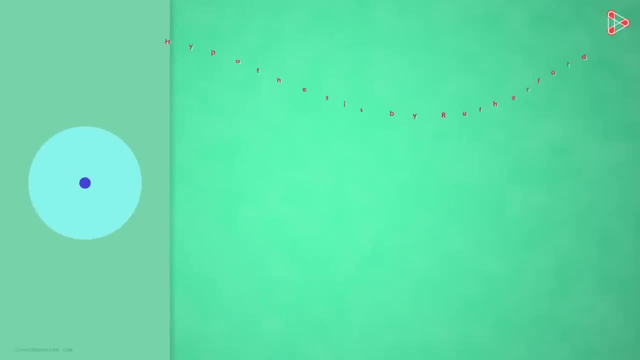 A few rays change their path and get deflected. Lastly, very few particles bounce back. These results compelled Rutherford to come up with a new nuclear model. Let's have a look at the hypothesis put forward by him. Firstly, there is a positively charged centre in an atom called nucleus.